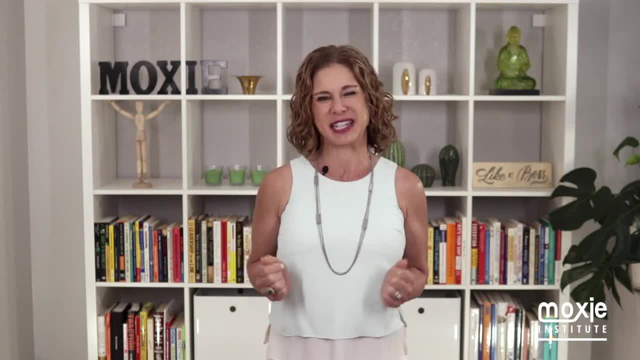 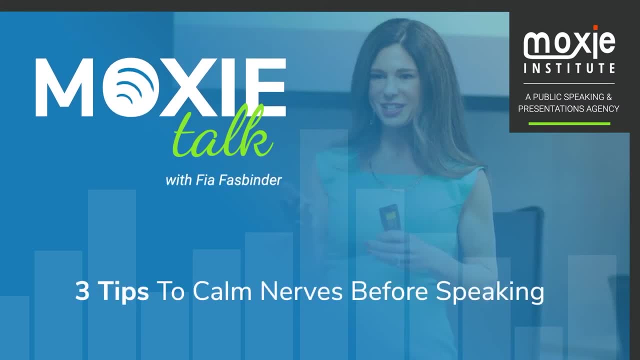 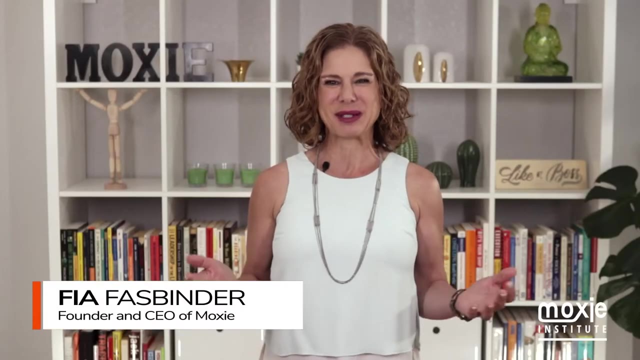 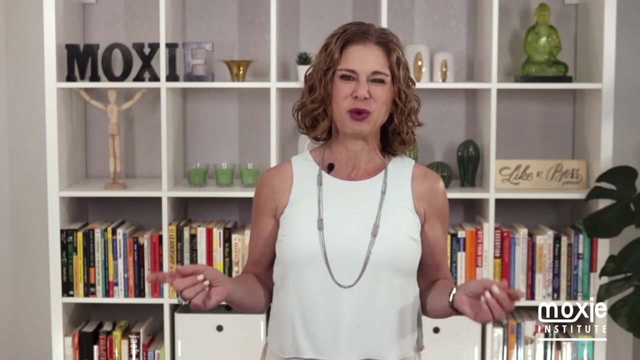 I am going to share with you my three favorite tips to calm your nerves before speaking. Hi everyone, I'm Fia Fassbinder and welcome to Moxie Talk, where we help you find your voice, share your message and lead with confidence. Today, I am going to unpack my three favorite tips. 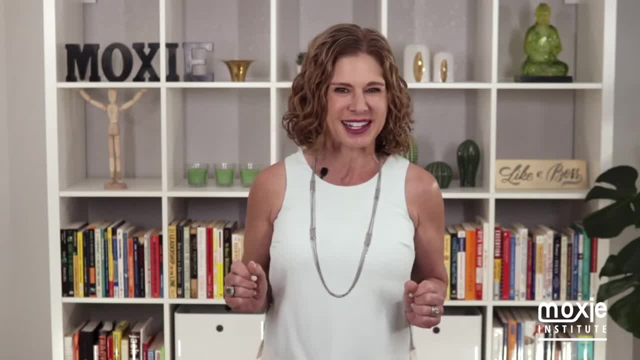 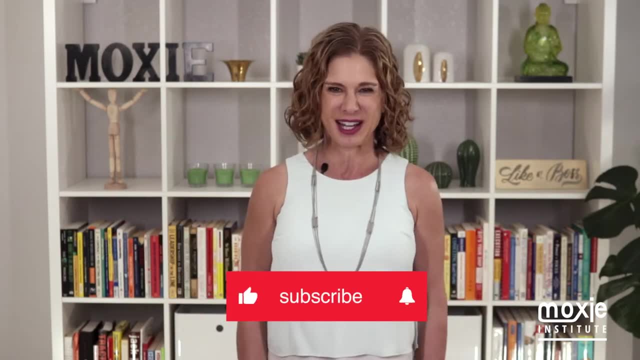 to calm your nerves before you speak. But before I do that, if you are watching me on YouTube, please make sure to hit that alert button so you get notified of all of the new content I put out. And if you enjoy watching my videos, please subscribe to my YouTube channel and hit that. 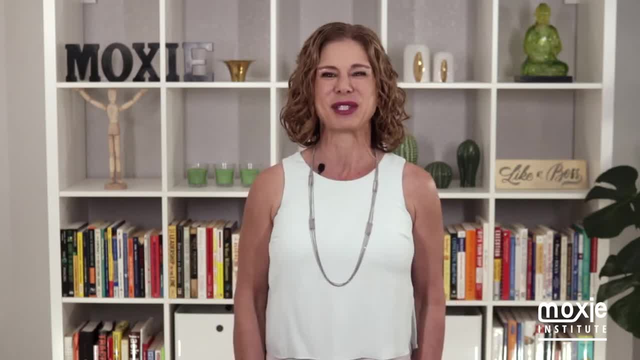 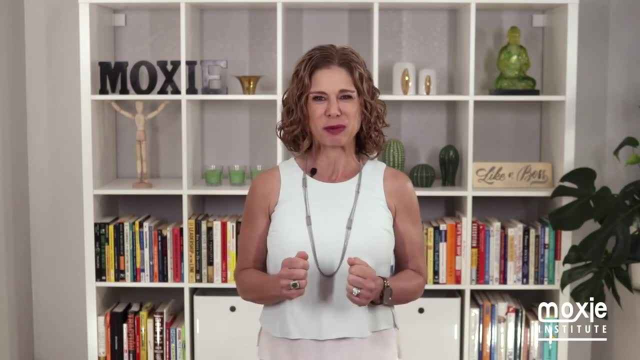 like button And if you enjoy this video, please make sure to share it, like it and subscribe to our channel. Studies on performance anxiety show that our heart rates are highest five minutes before a presentation and the first five minutes of a presentation. And why is that? Why do we get? 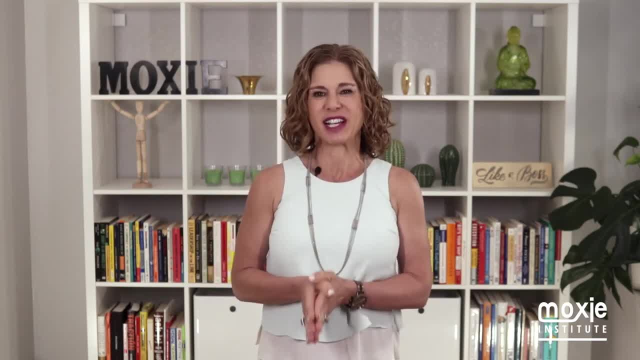 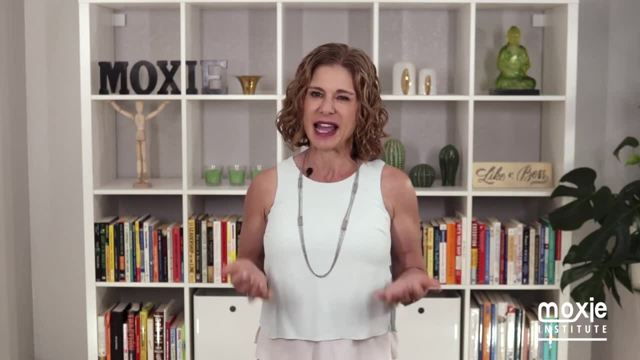 so nervous? Well, according to evolutionary psychologists, there are four factors. When these happen in combination, they trigger our body's natural fight or flight instinct. And these are the four factors that trigger our body's natural fight or flight instinct. And these are the four factors that trigger our body's natural fight or flight instinct. And. 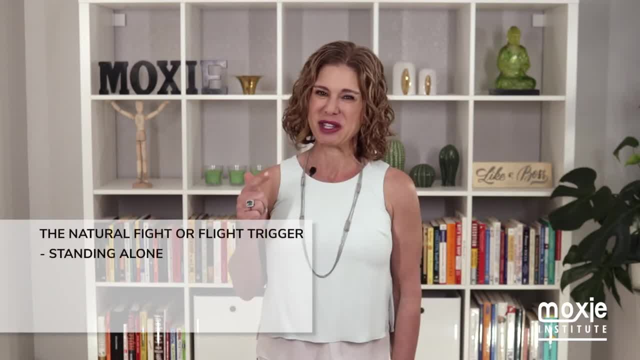 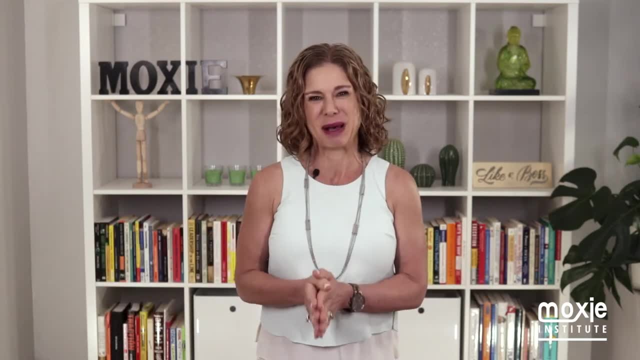 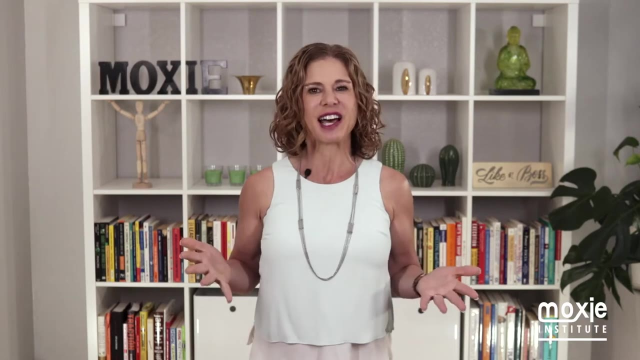 those four factors are standing alone with no place to hide, with no weapons and a large group of creatures staring at you. Sounds like public speaking right And if you are like most of us, you probably try to out-rationalize or out-logic your fear. But the truth is. 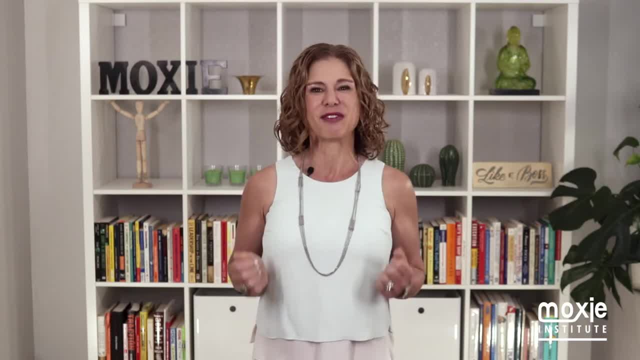 according to the last census study, more people are afraid of speaking than of death. Or, as Jerry Seinfeld put it, more people would rather be in the casket than delivering the eulogy. So if your brain tells you that it would rather be dead than be embarrassed, that's when you know your brain is. 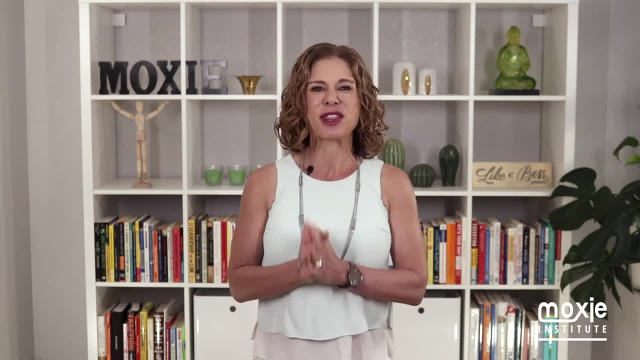 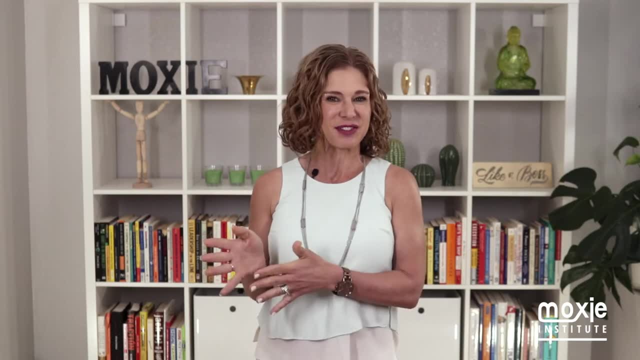 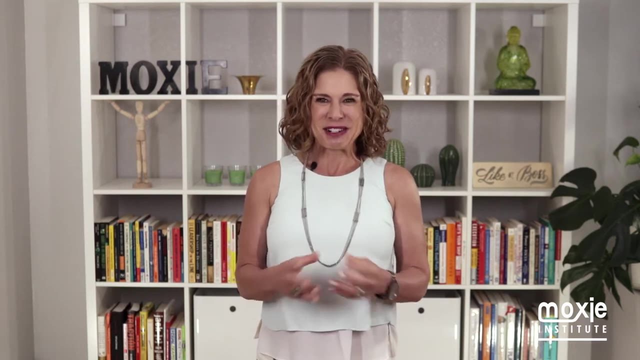 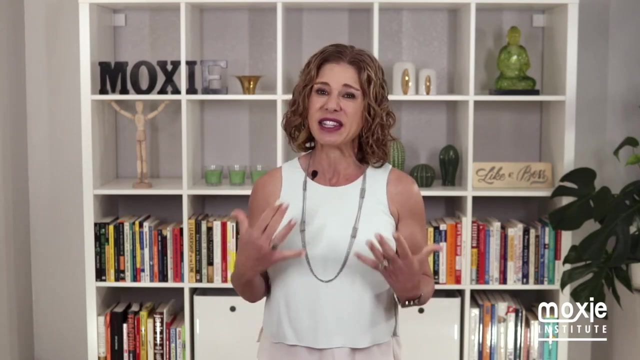 not working for you. So these are my top three tools, backed by neuroscience, to help your brain and your nervous system switch from fight or flight into rest and digest. Now, one known fact about neuroscience is that there are so many beliefs and ideas and methodologies, and 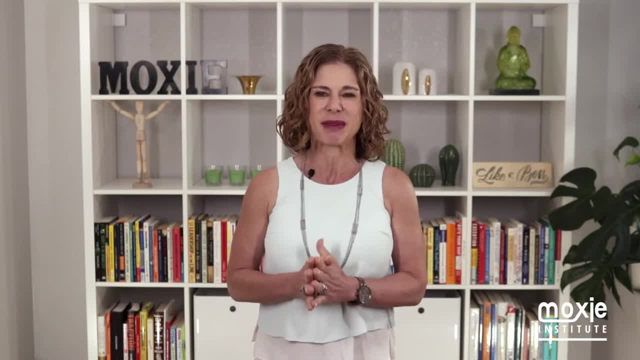 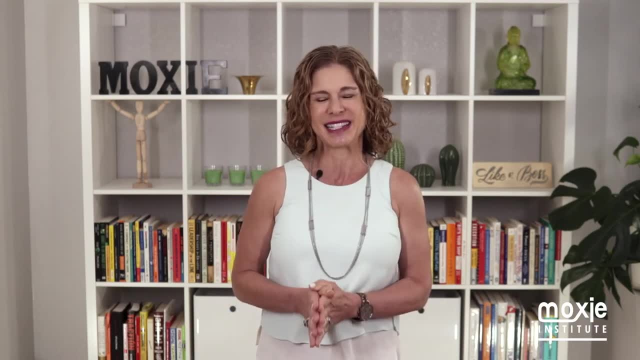 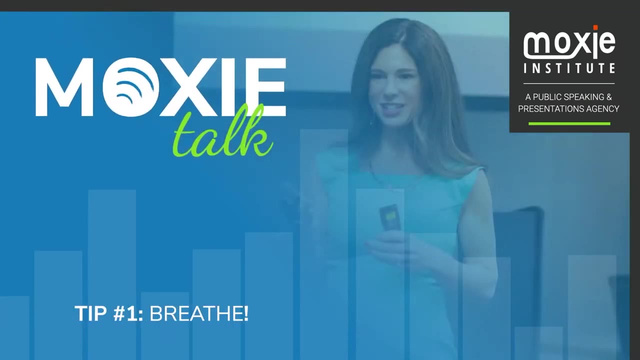 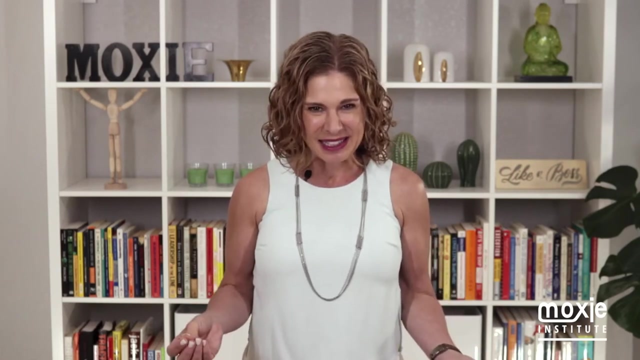 techniques that I've established over time and taught to my clients, And it is so wonderful to see those techniques backed up by studies in brain science. It gives legitimacy to what I know to be true and what I know works. So here we go. Tip number one: breathe. Breathing is your power tool for public speaking. You're 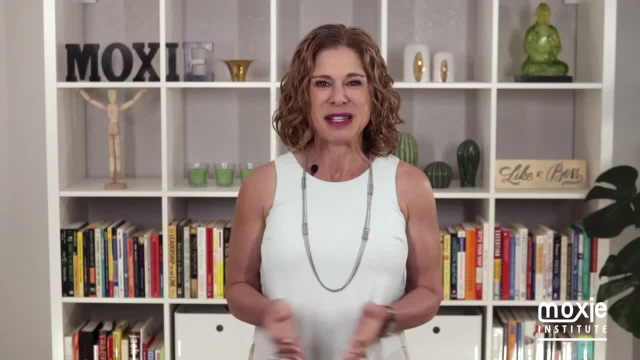 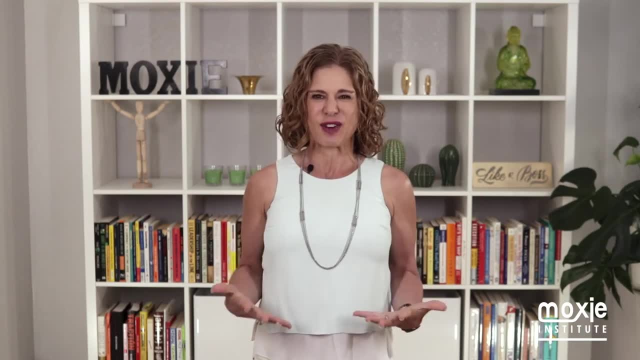 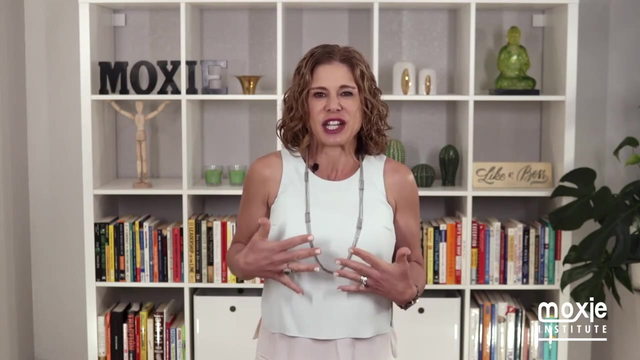 probably thinking I've been breathing my whole life, Fia, But the truth is you probably haven't been breathing correctly, Because when we experience stress, even at a very low level of fight or flight, we start to take short, shallow chest breaths. The biological reason for this: 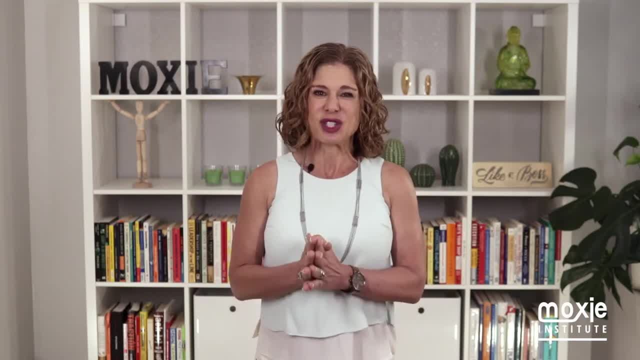 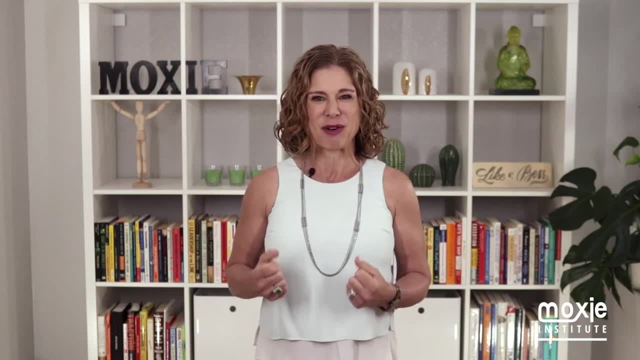 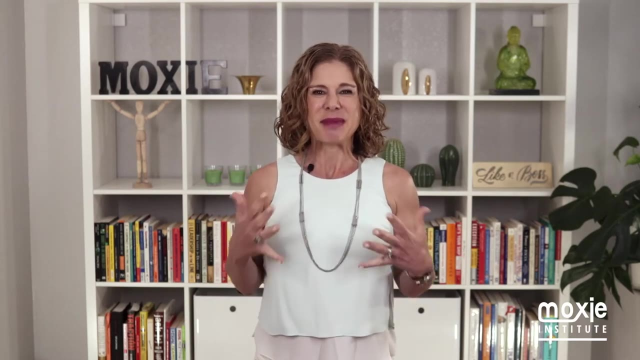 is pretty interesting. Our body is trying to protect our vital organs from being attacked And most of those vital organs are behind our diaphragm. So our diaphragms tighten to protect our vital organs from being attacked. But to make this more practical, breath is directly tied to 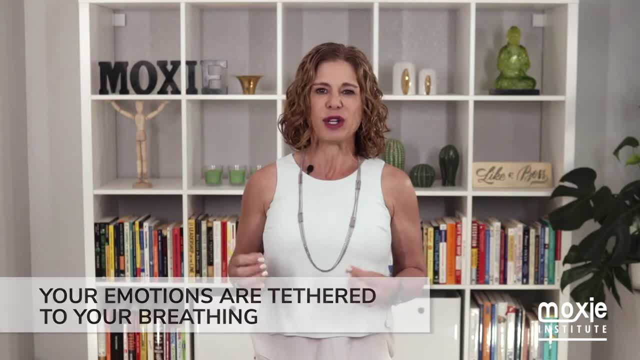 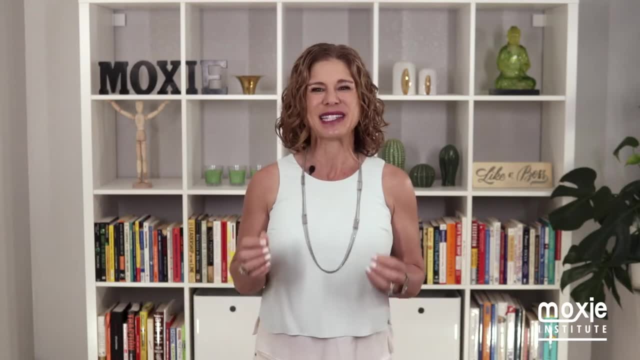 emotion. Think about the difference in your breath when you're crying or you're stressed out versus when you're fighting. The great news is that we can manually control our breath and use it to control our emotions. Breathing correctly can get us to experience the same calm and zen state we feel before bed. 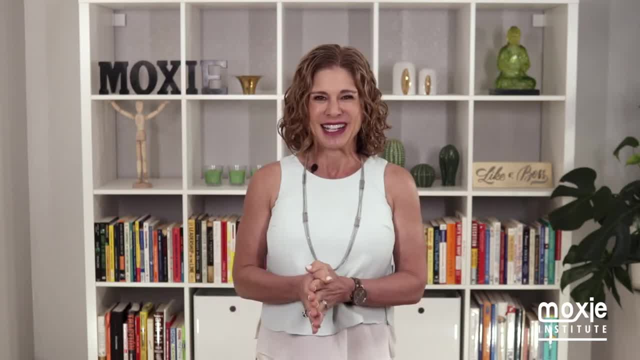 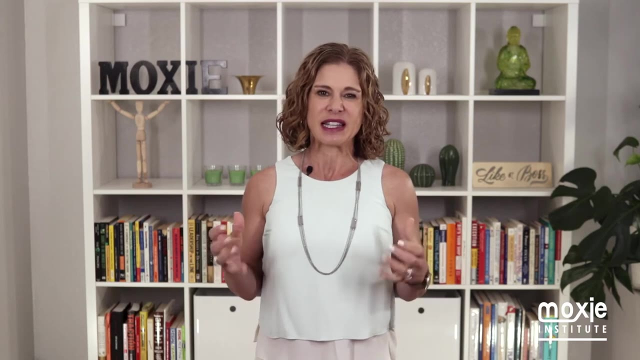 even when we're about to do a presentation. Now there was a cool study recently published in Sydney, Australia, where they taught the entire Philharmonic Symphony performers to breathe from their diaphragms And then, before a performance, they hooked them up to electrocardiograms. Now, as soon as these. 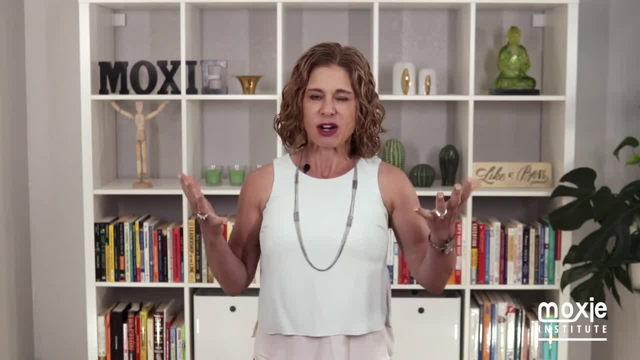 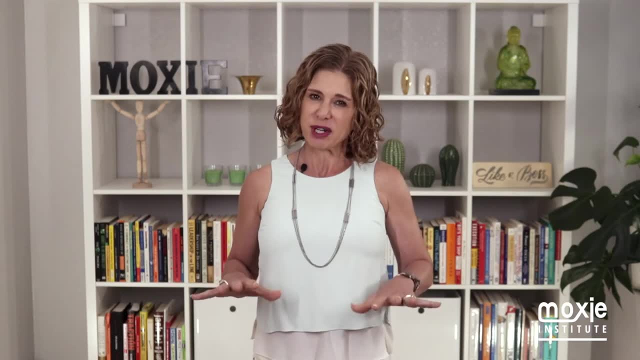 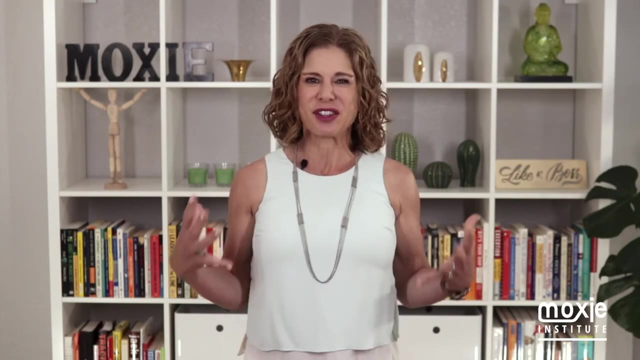 performers started to use diaphragmatic breathing, their heart rates subsided, So they were able to go into that performance with the low heart rate of a person that is falling asleep. So the study went on to say that, aside from beta blockers or other techniques that are so expensive, breathing 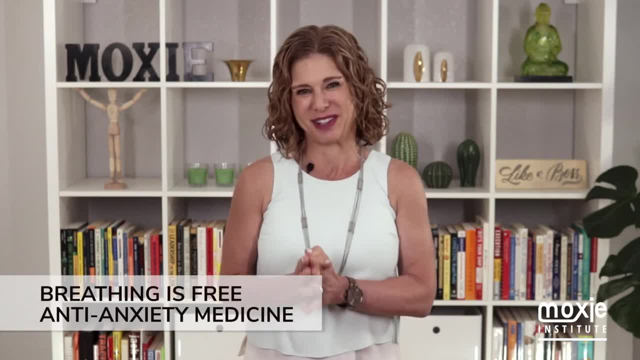 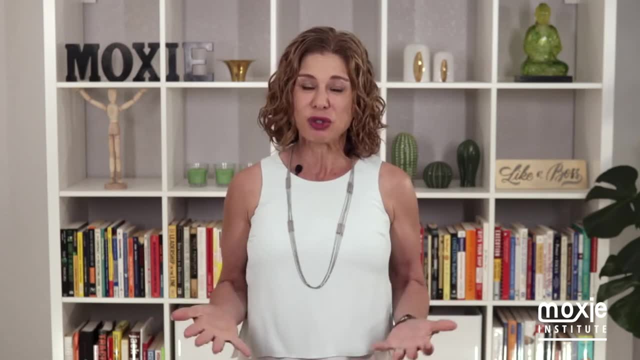 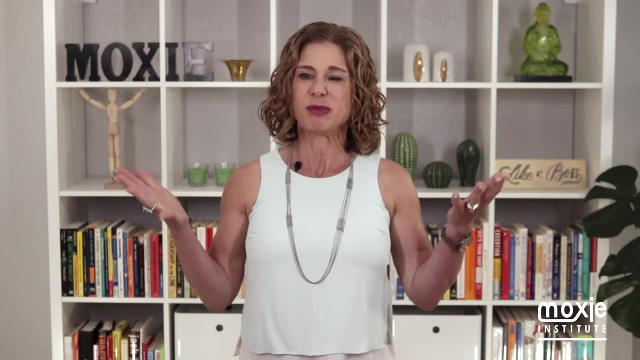 is free. It's the cheapest way you can calm yourself down And breathing isn't a woohoo thing anymore. In fact, they are teaching diaphragmatic breathing to soldiers in boot camps because this is something that they only need their bodies. They can do it in battle and it can subside. 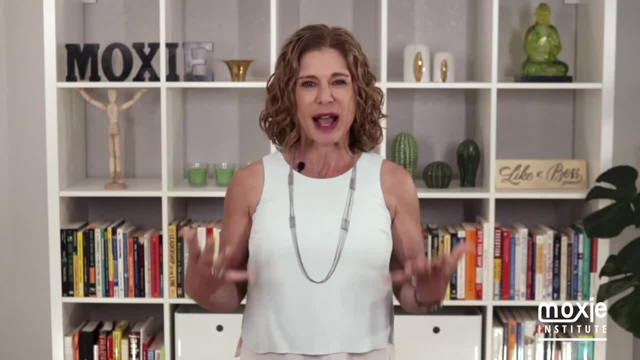 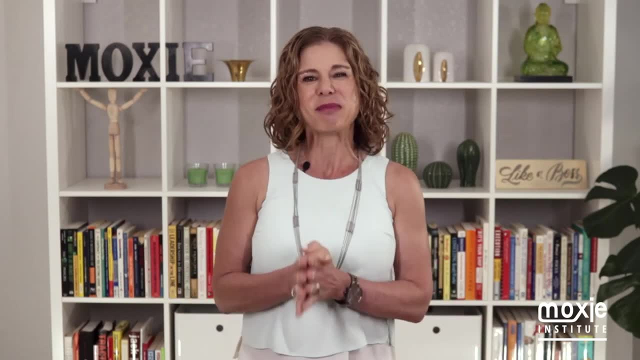 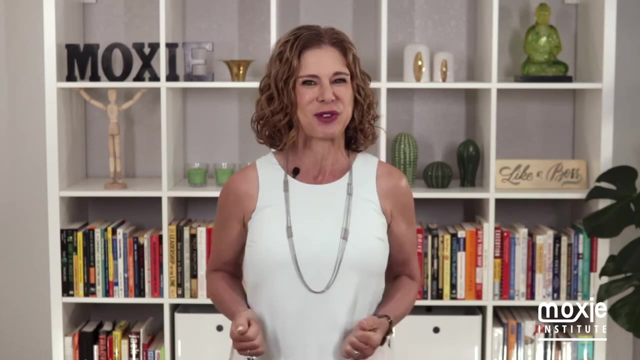 their heart rates to a level where they can make rational, calm decisions. So how do we do this whole breathing thing? We do it by using our diaphragms, And for those of you who haven't watched my previous videos, I'm going to give you a crash course. 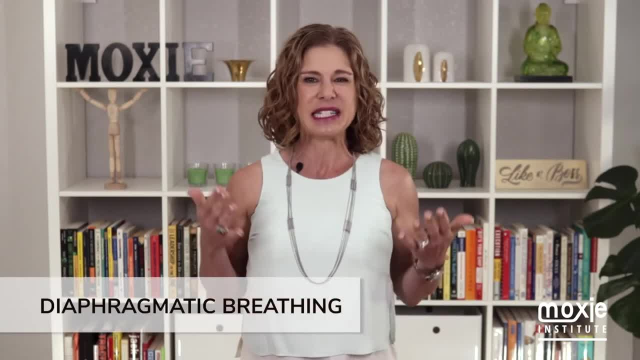 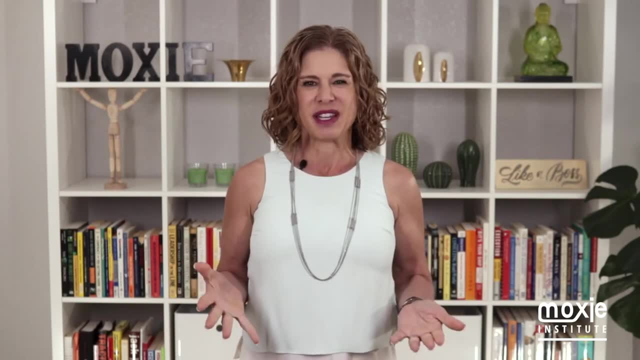 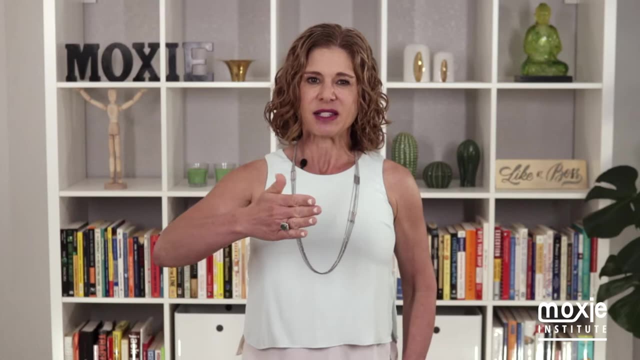 on all things diaphragmatic breathing And if you want a deep dive into anything around breath support, check out my previous videos. So what is your diaphragm? Your diaphragm is a sheath of muscle that sits between your chest and your abdomen And it's dome-shaped And its whole purpose: in your body it goes. 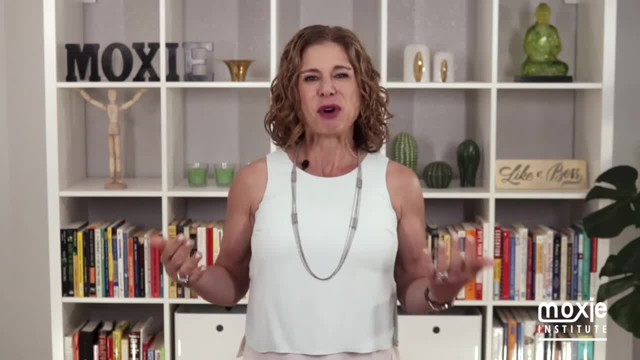 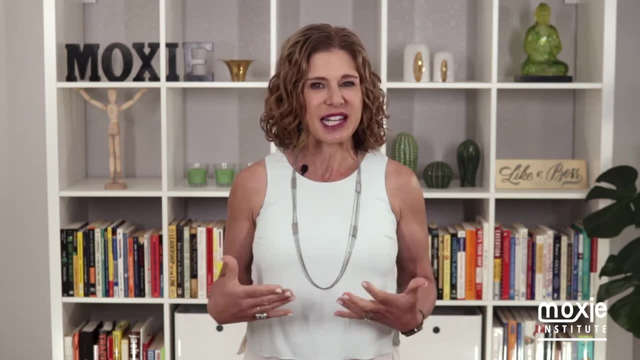 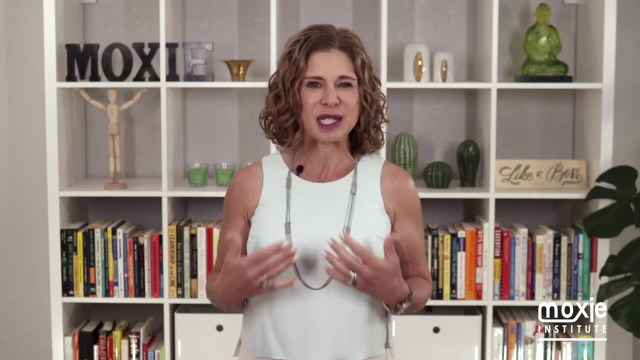 like this, and it pushes air in and out of your lungs. For most of the time, our diaphragm lays dormant. However, when we get stressed, like before a presentation, we need the extra air and the extra oxygen to calm us down, And we can do this simply by breathing in. 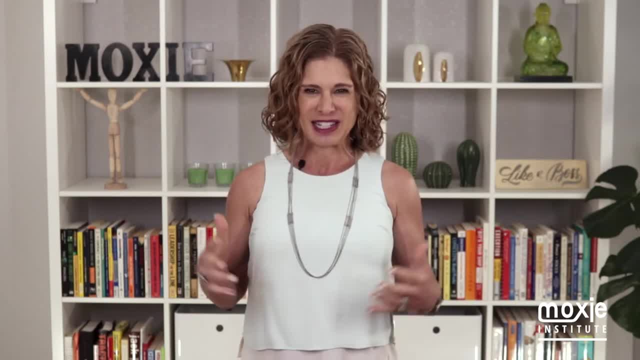 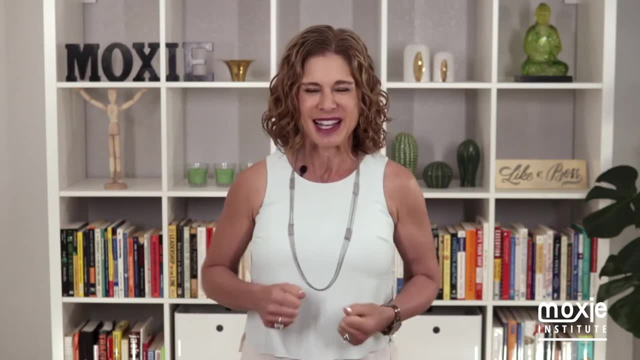 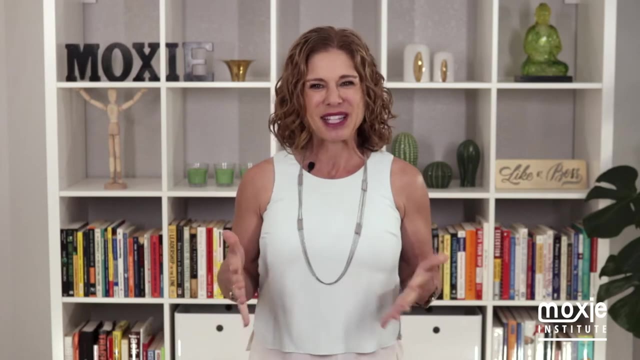 a pattern that I call low and slow, to flood our body with extra oxygen, increase our blood oxygen levels, which in turn lowers our heart rate and causes a really cool domino effect of hormone release. to help us calm down, And speaking of hormone release, with diaphragmatic breathing- we can all be alchemists to our 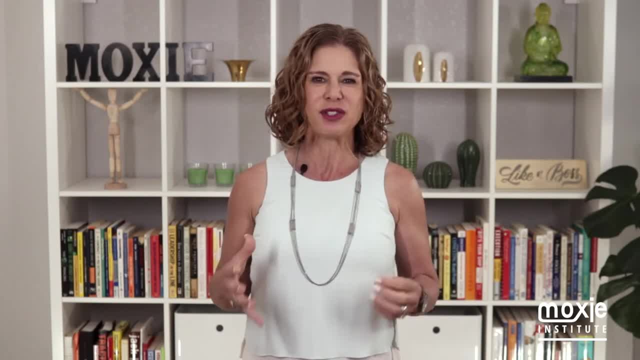 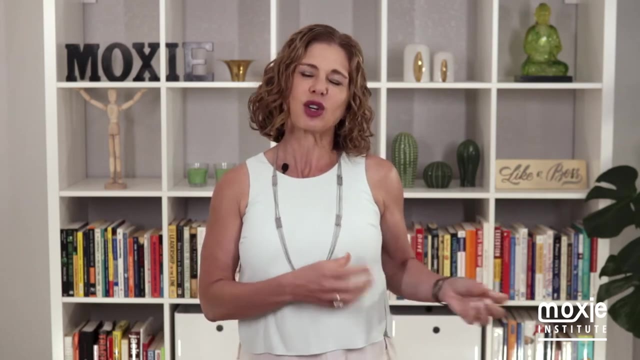 own biochemistry. It is so cool When we learn to do this. by breathing correctly, we can literally change our hormones. We can alter our biochemistry by sending signals to our neurotransmitters that we can release the fight or flight mechanism and secrete more. 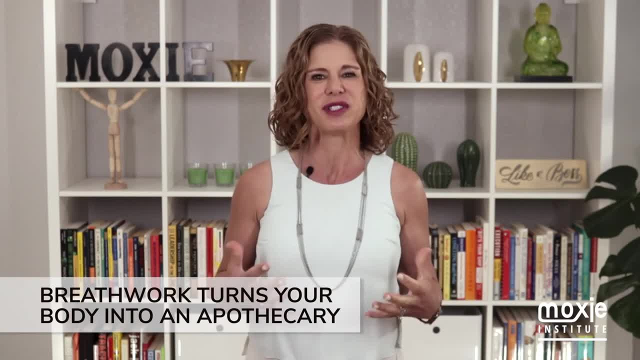 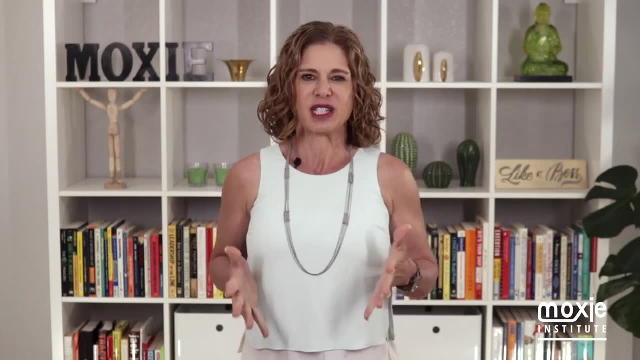 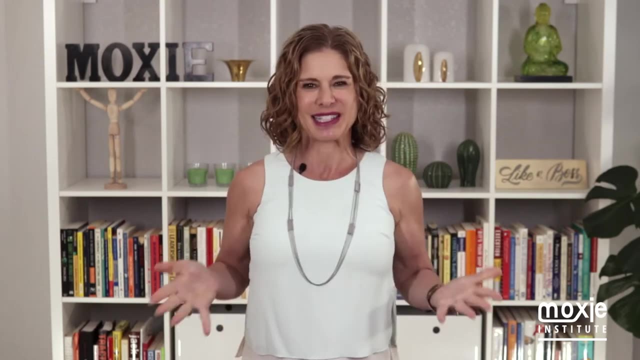 dopamine and serotonin, those feel-good hormones that put us into rest. So we literally are manually switching our nervous system from sympathetic nervous system to parasympathetic nervous system. So how does this happen? The diaphragm was designed to send messages to your brain about 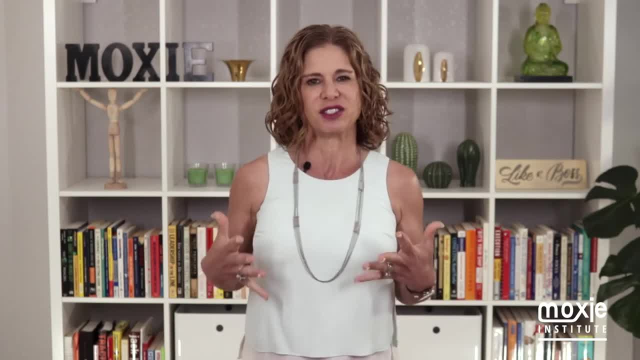 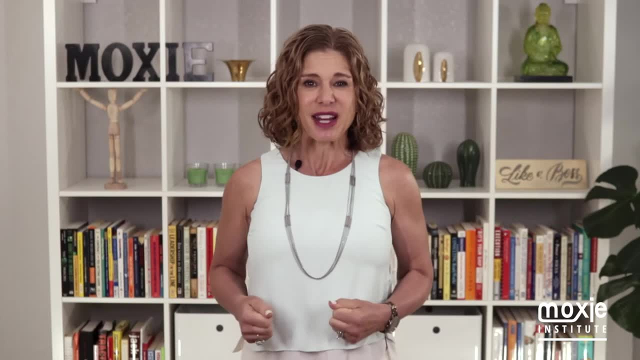 the status of your body, And it does this through the vagal nerve. So if you breathe fast and rapidly because you're panicked, you're sending messages through your diaphragm to your brain that, hey, we're moving, and really fast, we're running, we're probably 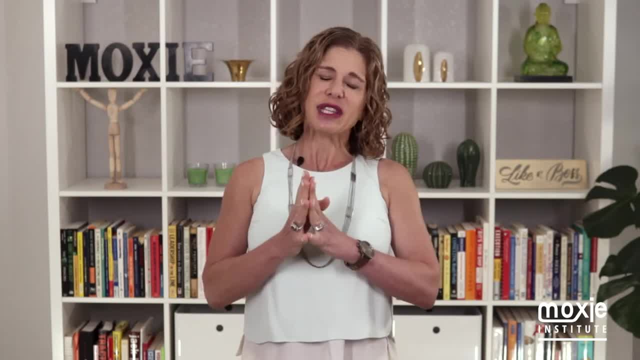 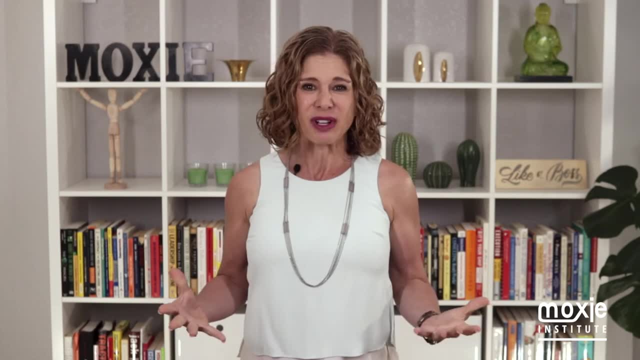 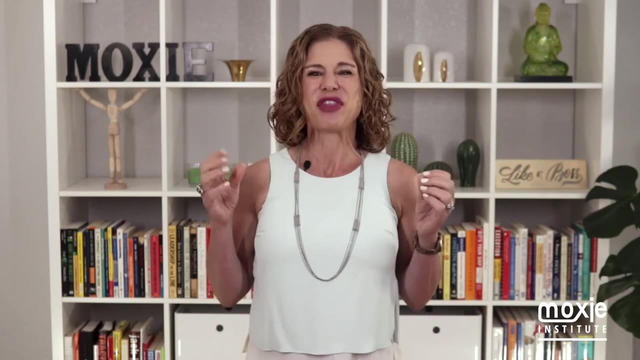 running away from something that's going to eat us, And if you breathe slow and low, you're sending messages to your brain that everything is cool and we're probably no longer being chased by that thing that was going to eat us. So, now that I have thoroughly explained the neuroscience behind diaphragmatic breathing, 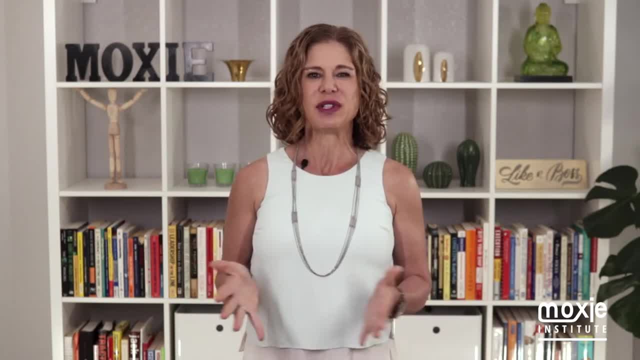 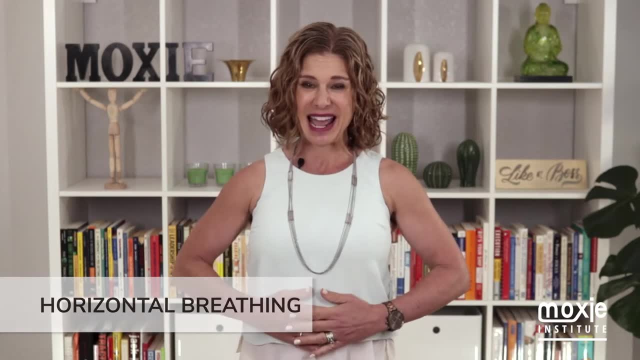 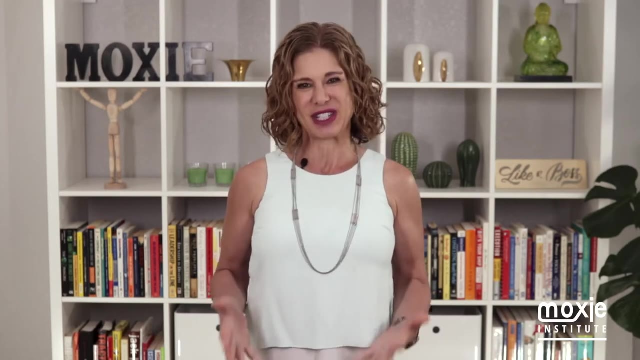 let's learn how to do it Now. I refer to diaphragmatic breathing as horizontal breathing, because we are going to breathe in and out, as opposed to vertical breathing, which is up and down, which is what most of us do when we're stressed or we hold our breath. 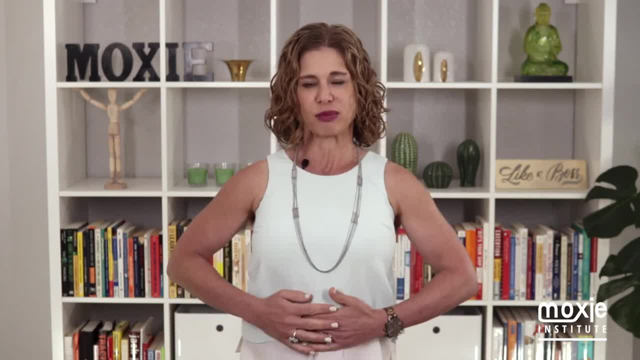 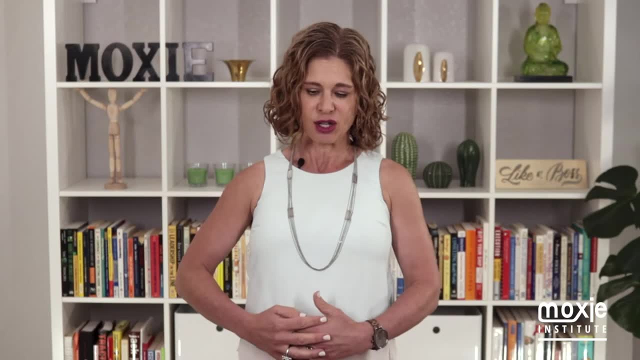 So, in order to practice our horizontal breathing in and out, let's imagine for a second that you have a balloon in your belly And every time you breathe in, you feel the balloon balloon up with air and it pushes your belly out. and every time you breathe out, 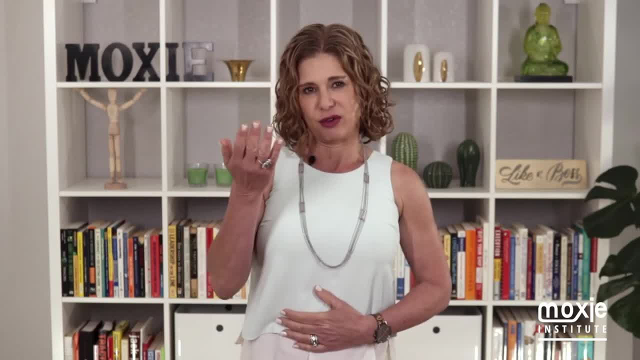 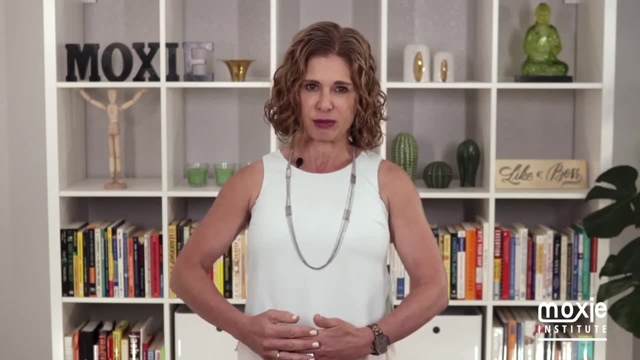 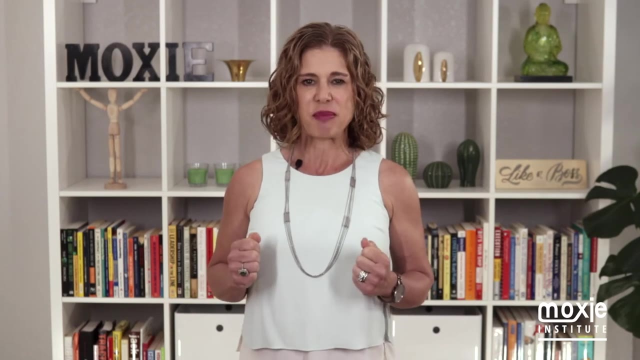 you're all that air goes out your balloon and out your nose and mouth. so notice, you're going like this: in and out. you're filling up your balloon, you push out, you're letting the air out of your balloon. it goes in. it's literally that simple, and now you just have to do it in a pattern of four, four, six. we are going. 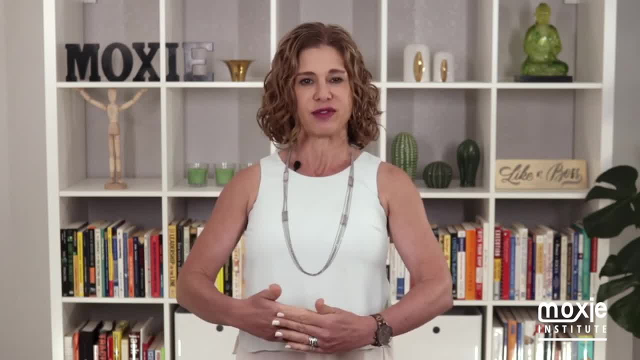 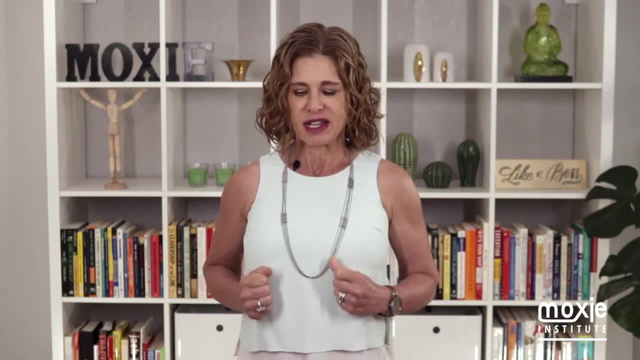 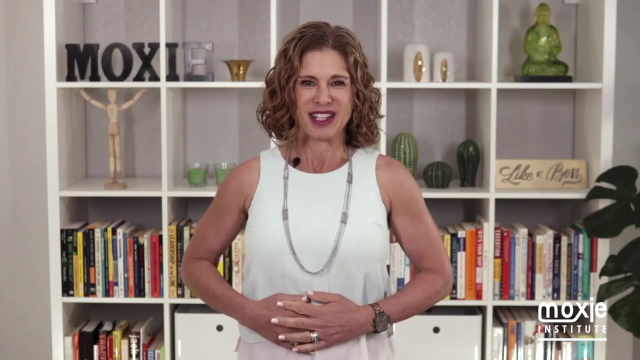 to breathe in. fill up our balloon for four seconds, hold it for four seconds and breathe out for six seconds. now, the reason I have you breathe out for longer than you breathe in is the more you exhale, the more you will inhale, and we want to flood our bodies with all that good oxygen. so in for four, hold for. 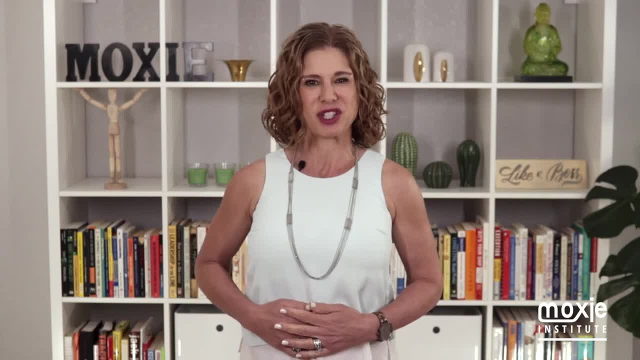 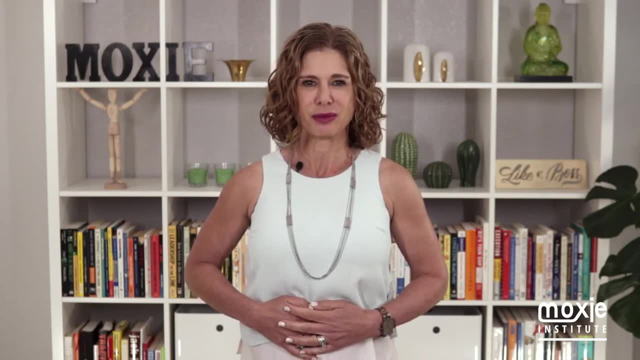 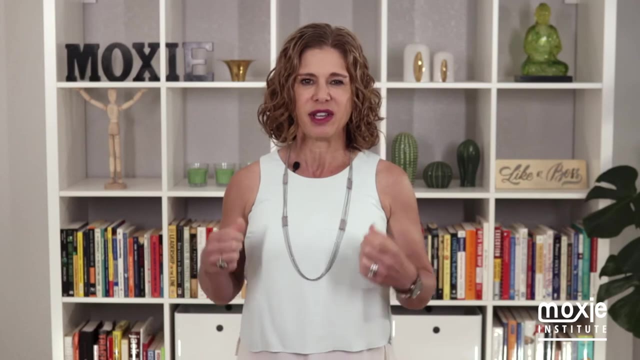 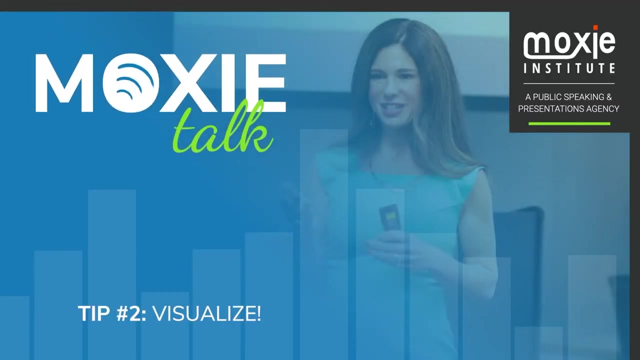 four out for six. I'm going to demonstrate it once it looks like this, that's it. do this: four, four, six breathing pattern as many times as you want to calm down. you will literally feel your heart rate subsiding and yourself coming back down to planet earth. 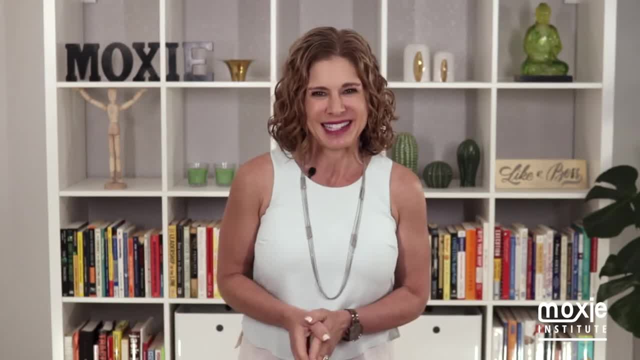 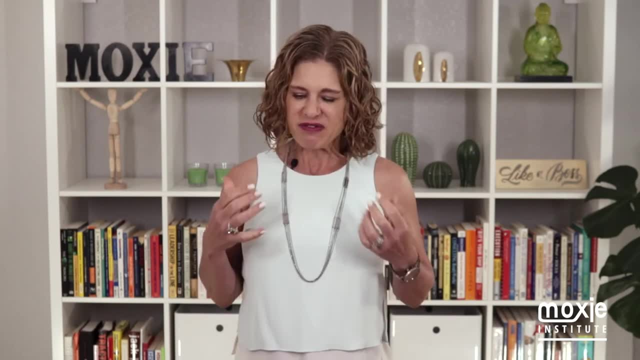 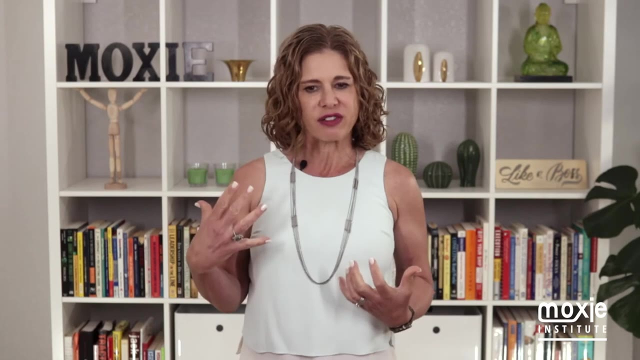 tip number two: visualize if I have to do a presentation or my clients have to do a presentation that they're really nervous about. we visualize ourselves going through every detail of the presentation: what we're wearing, the look on our face, the stage we're presenting on, how we're walking, the 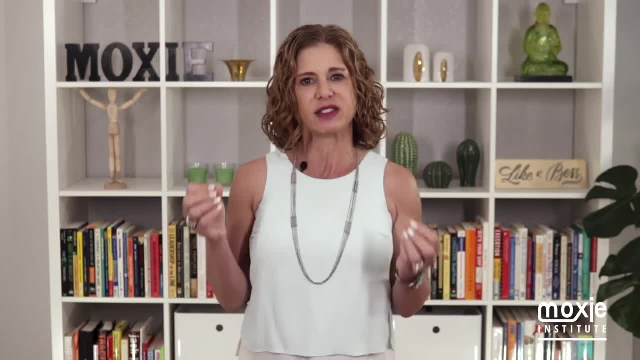 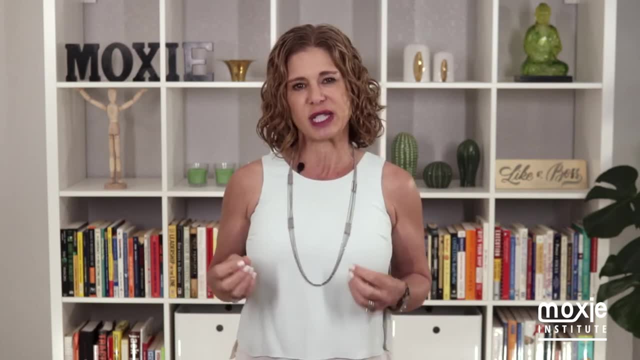 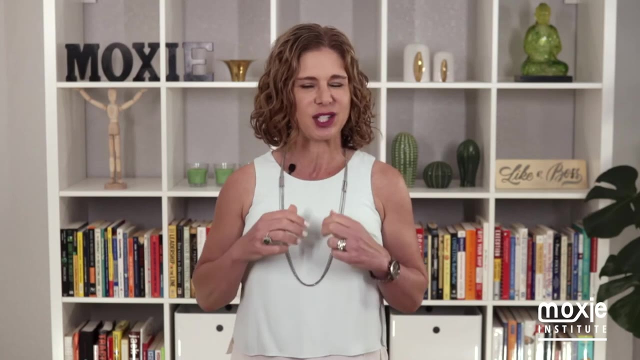 sound of our voice, the smell in the room, every single detail, and there is neuroscience behind visualization. the brain doesn't know the difference between doing something and visualizing it, so this is a perfect way to practice having a super successful experience without actually doing it. you can. 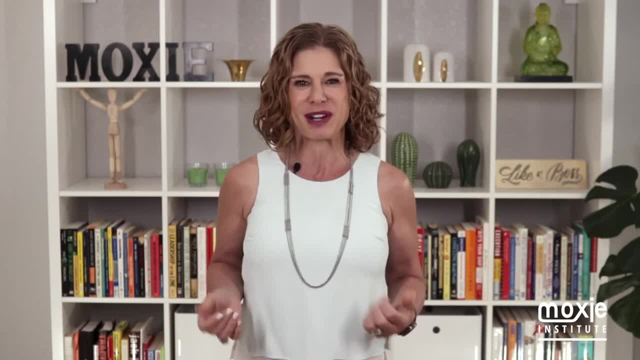 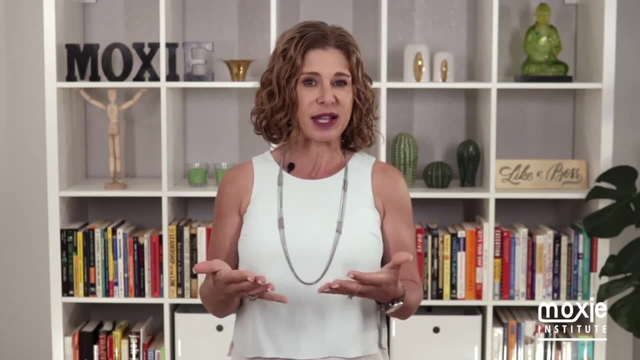 convince your brain that you've already done this great thing, that you're going to try and do to get better at it. for you done this great presentation. It is literally a brain hack, because your brain uses the same neuropathways if you do the thing as if you visualize it. That's why athletes have been 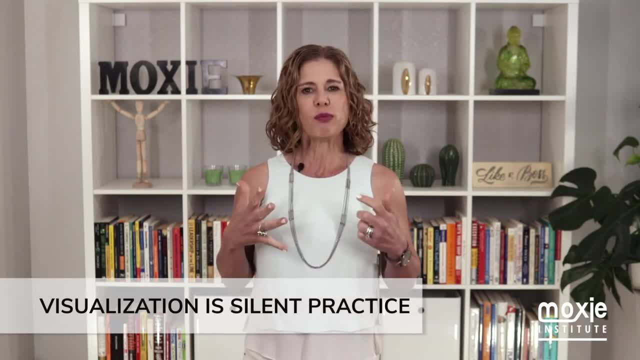 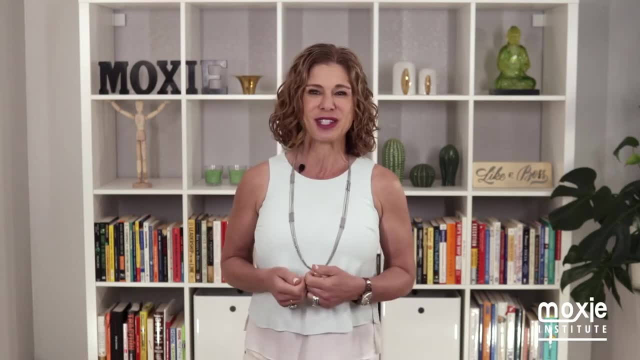 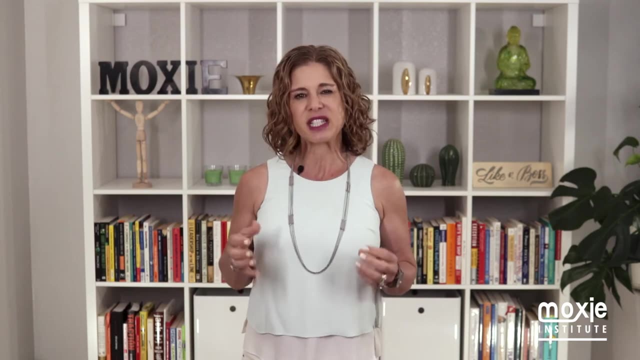 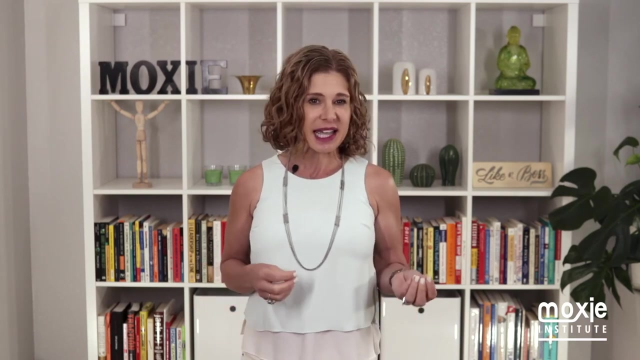 using visualization for so long. There's also multiple studies that have shown that people who visualize themselves delivering a smooth talk perform better than those who don't. In a recent study in Psychology Today, results revealed that performance visualization, which is what we're doing here, was generally more effective than other interventions like medication or yoga, or 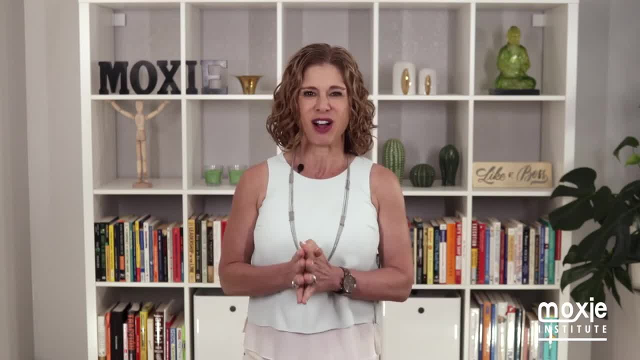 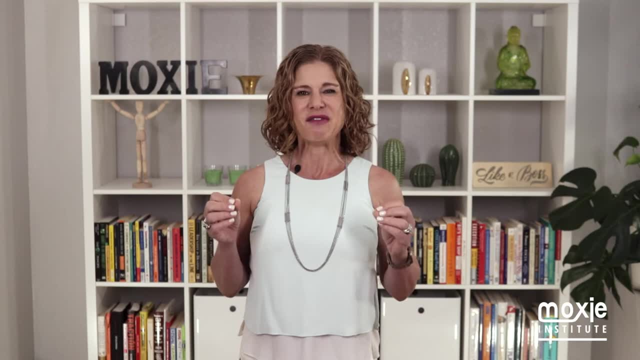 pre-presentation warm-ups. It was more effective than all of those for reducing self-reported negative thinking. Now, what does this mean? It means that visualizing a positive performance is the antidote for a negative thinking. It means that visualizing a positive performance is the antidote for a 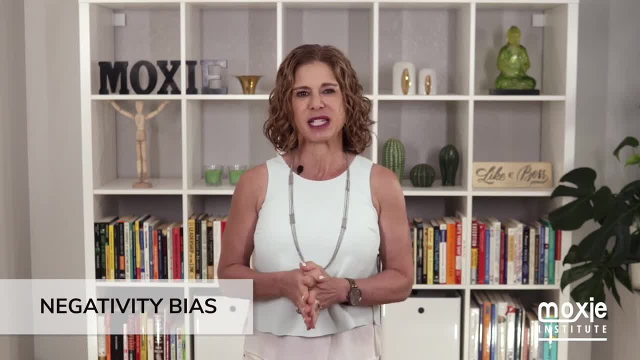 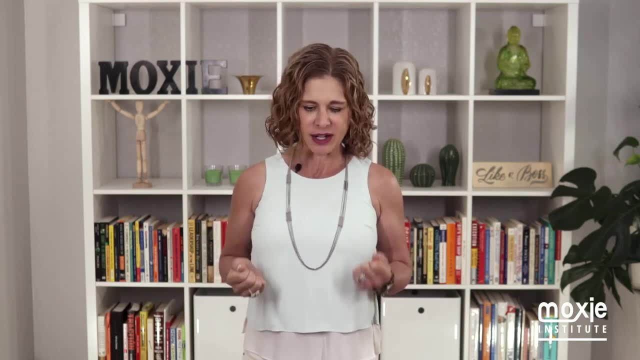 negativity bias. Now, I've spoken about our negativity bias before, but for those of you who aren't familiar with it, our negativity bias is our hardwired, innate inclination to hang on to negative experiences more than positive experiences. Negative ones are like Velcro. 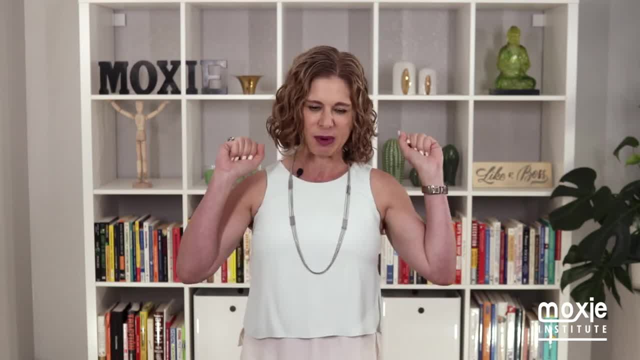 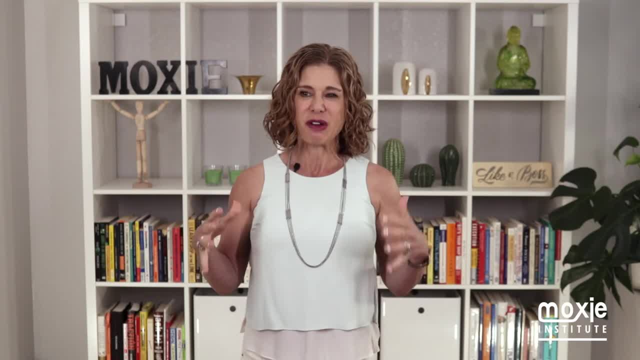 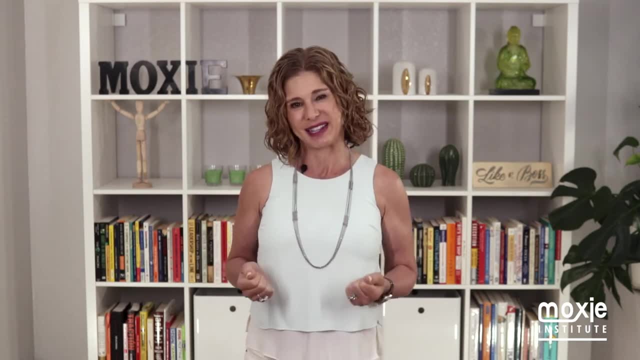 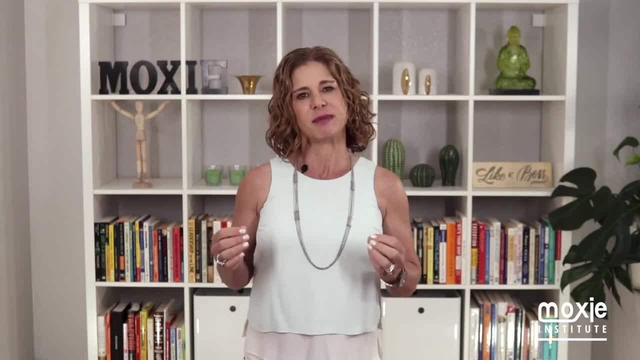 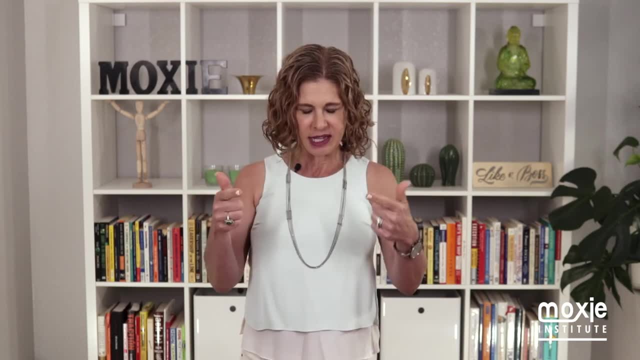 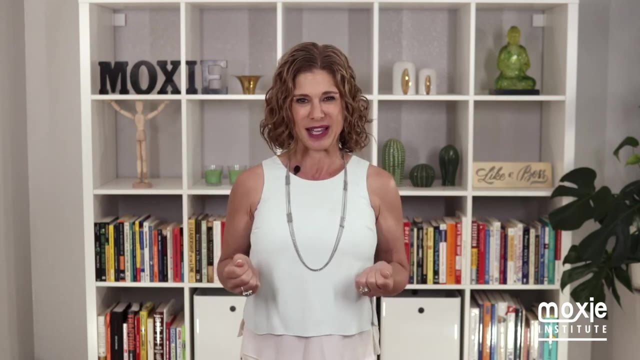 before any Olympic event And he visualizes himself swimming through the water through his own eyes and seeing himself win through his own eyes. And then he visualizes himself from the view of the people that are in the stands watching him swim and win. And he does these two. 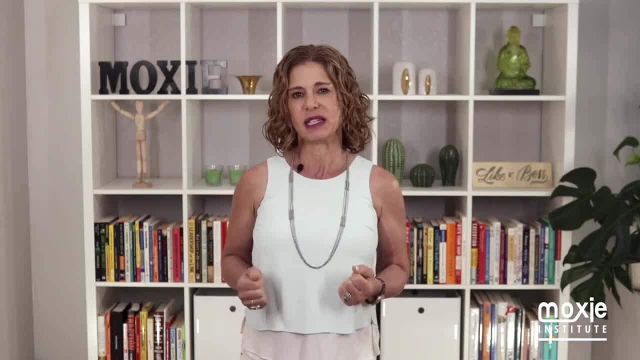 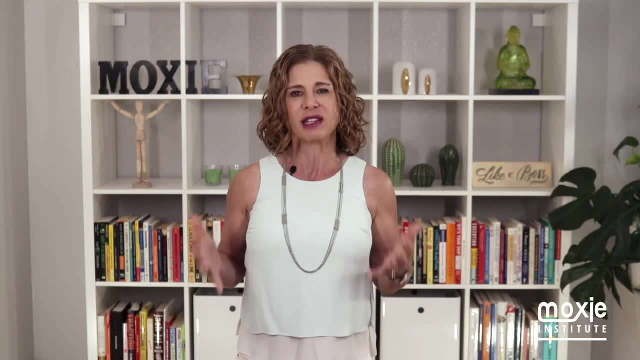 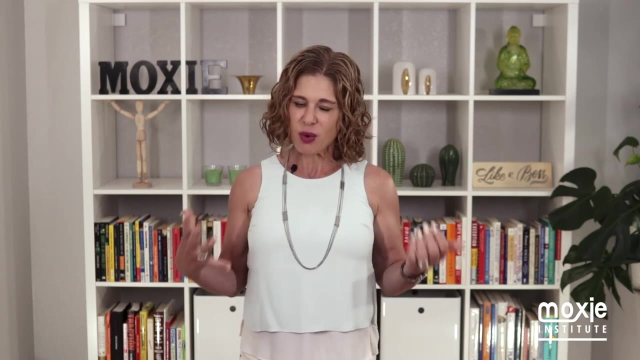 visualizations every day for a month before the Olympics And he credits this to his success. It is one aspect that he uses that sets him apart from a lot of other performers and athletes. So next time you have a presentation before it, right before, visualize this presentation going just stunningly. 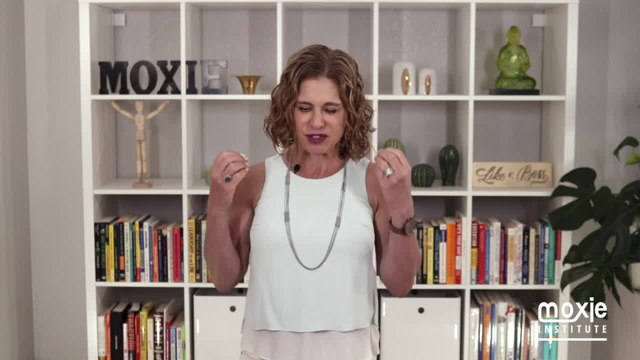 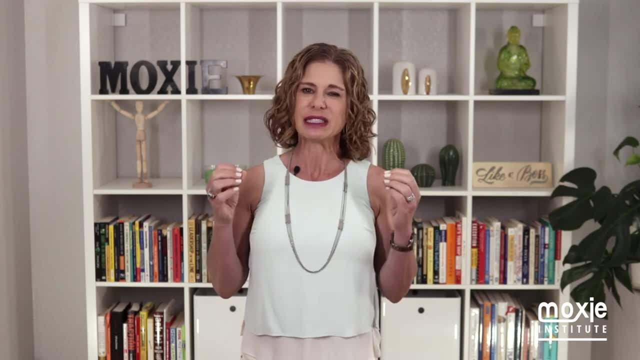 swimmingly. When you're crushing it, everything that you have to do in your mind go through it and go through it as if you were having a successful presentation. You will trick your brain into having a rock star presentation before you actually do it. 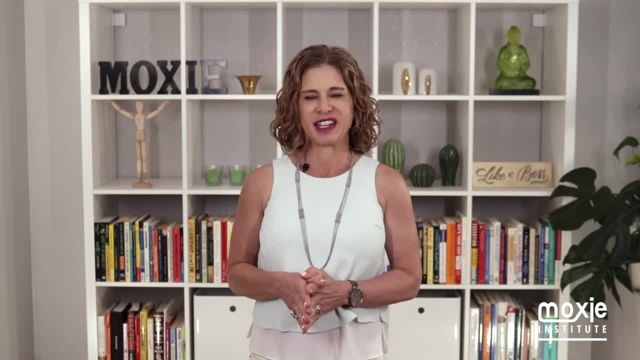 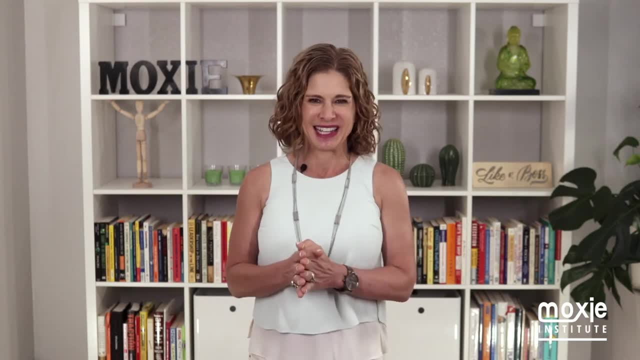 Tip number three: create your own mantra. Now we all have both a negative self-critic and the best coach we've ever had inside of us, And this has been proven by recent research that came out of Georgetown University that said that. saying something. 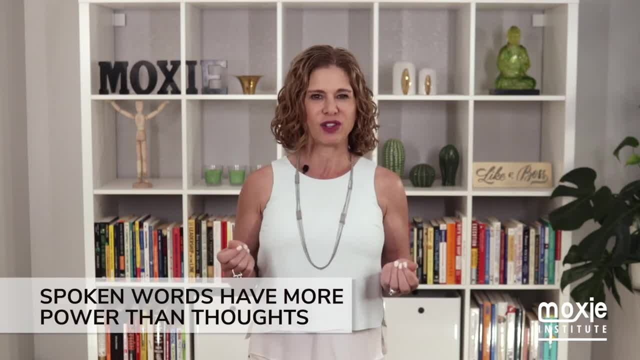 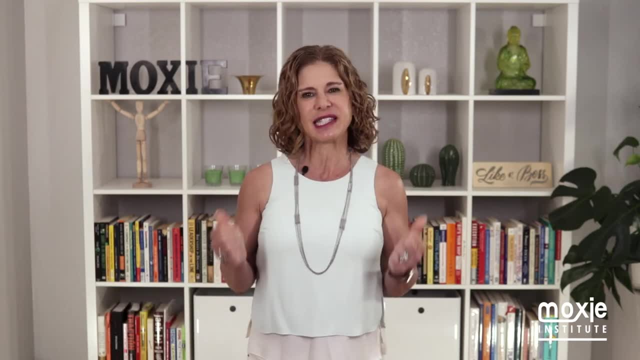 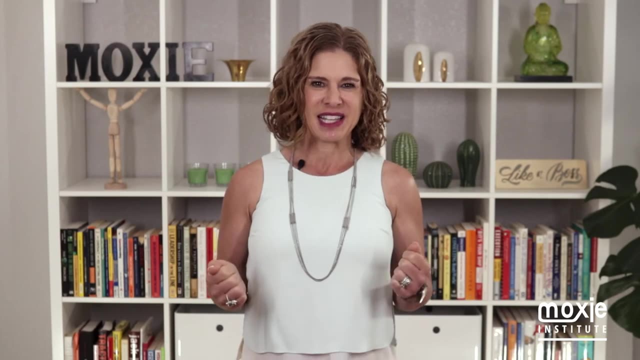 aloud is 10 times more powerful than saying it in our head. And negative things- negative sayings- are four to six times more powerful than positive ones. Now, we just spoke about our negativity bias. This means if you say something aloud like I'm dreading this, 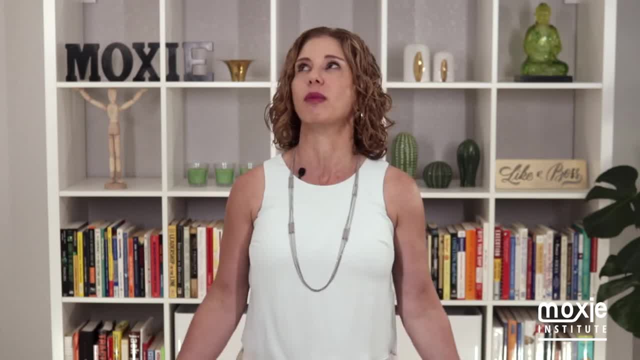 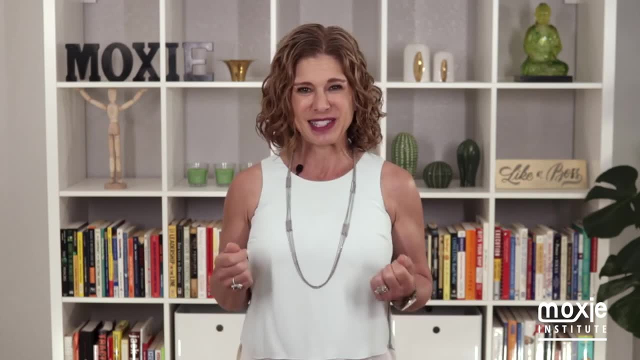 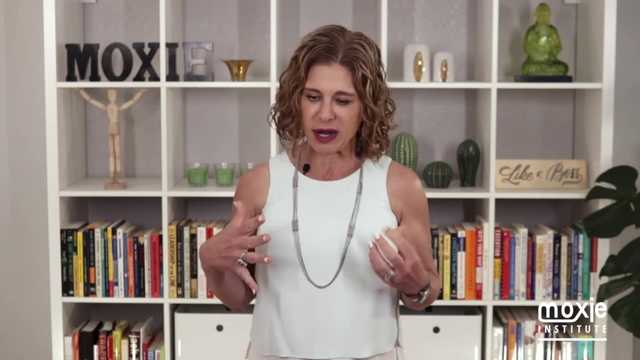 presentation, or I just suck at public speaking, or this is so miserable. You are 40 to 60 times more likely to create that result for yourself if you say it aloud and you say these negative things. So what we need to do in these kind of situations before a presentation, when we're feeling the 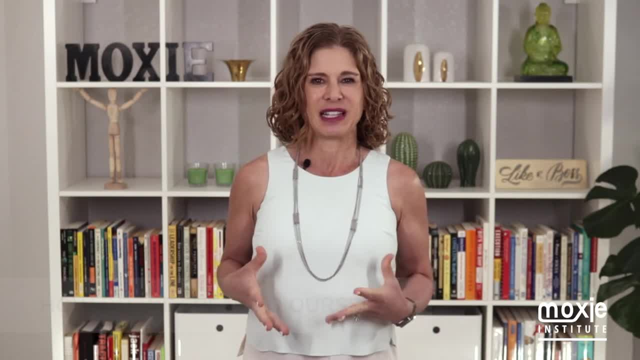 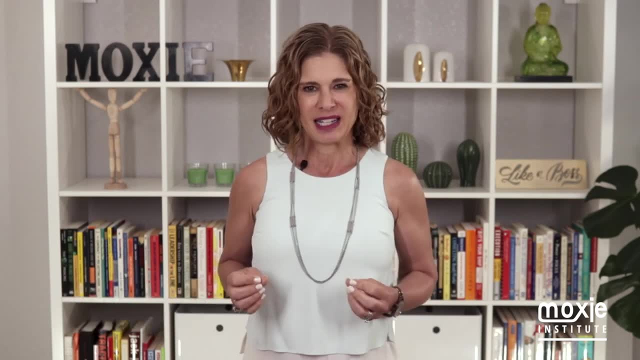 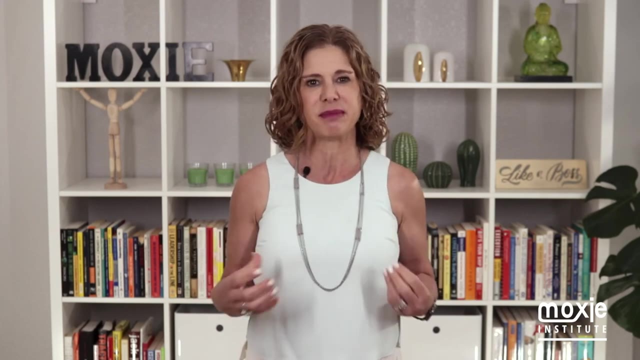 nerves is to ask ourselves: how do you speak to yourself, especially in those stressful or difficult times? Now a lot of sports psychologists and sports psychologists to very important teams in the NFL and the NBA players have them do an exercise called the microphone exercise, and I 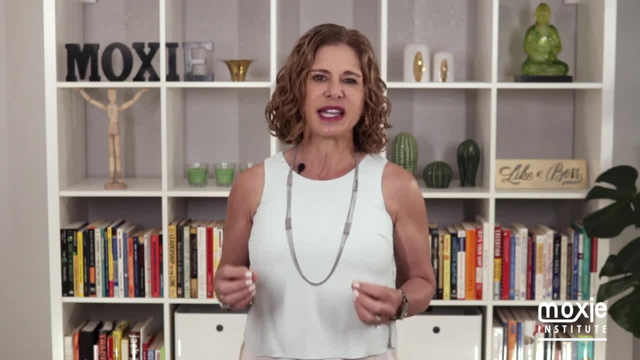 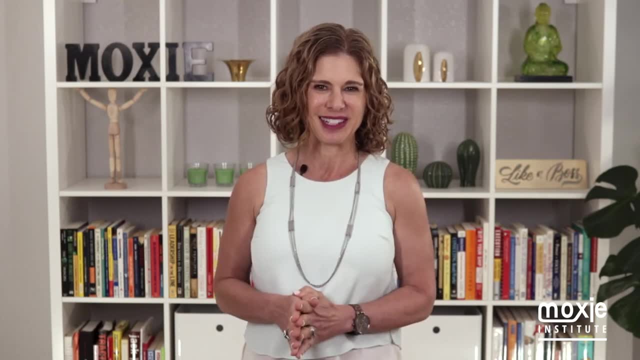 really love this one. Imagine that you are holding a giant microphone and I want you to listen to the voice that's coming out of the speakers linked to that microphone. Just take a step back and observe and hear that voice. What is it saying? 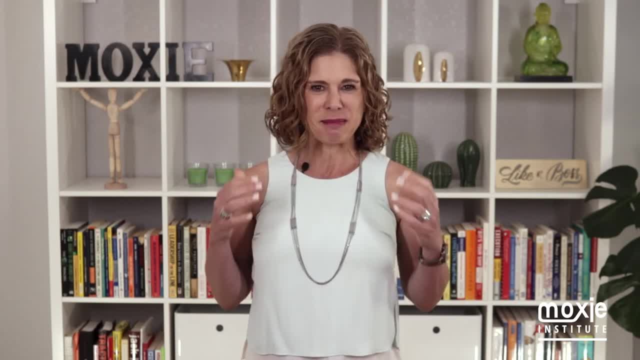 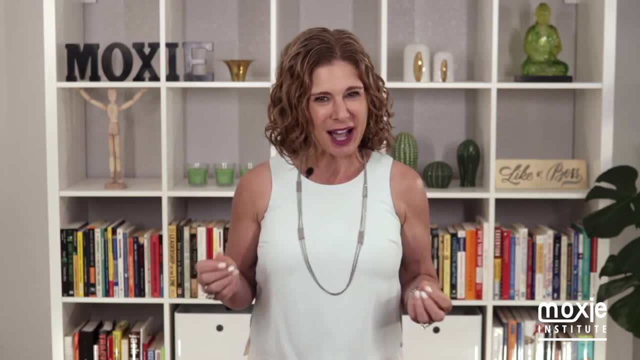 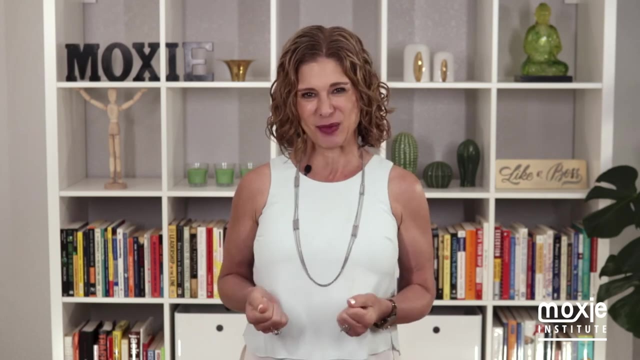 Now ask yourself: would you want that message to come out of a megaphone, a Megatron, for a crowd of people to hear? Would you be proud of that messaging? Probably not, But despite that, we still continue to talk to ourselves this way. So it is really up to us to turn down the volume on the 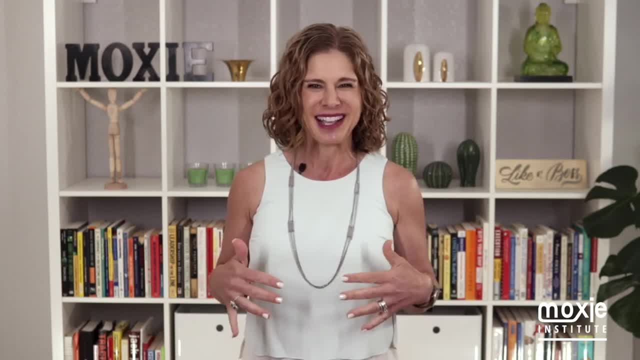 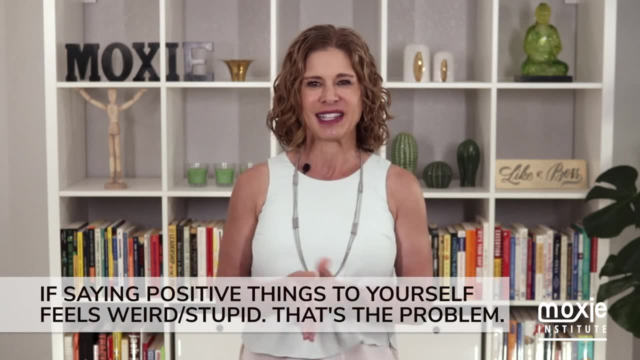 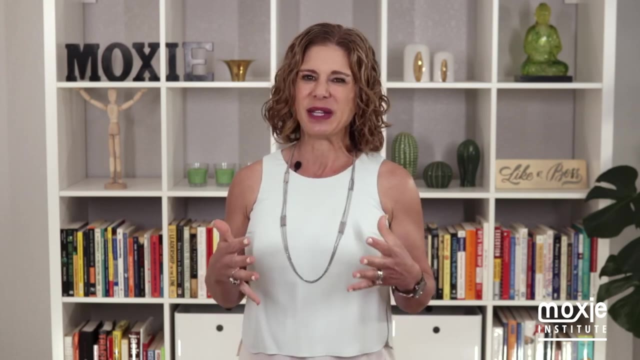 mic, with the, with the naysaying voice, with the hater, and turn up the volume on the voice of the coach that has a belief in us and a belief in our abilities. And we can do this by creating a mantra that we can get behind. Now, once we do that, we need to read it, we need to write it down, we need 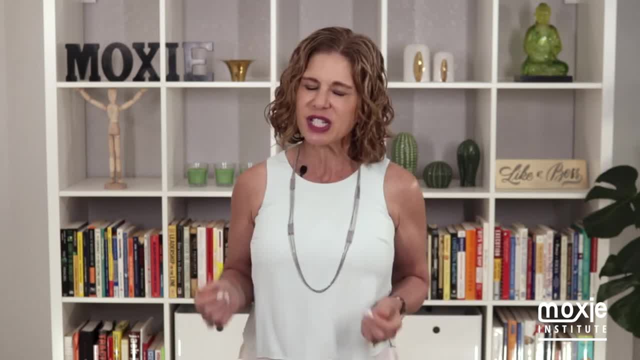 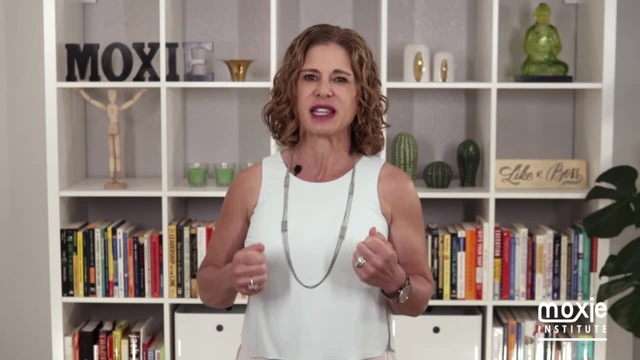 to test it in a variety of stressful situations, so it works for us when we most need it And we need to keep refining it until we come up with a mantra that feels like the best coaching moment we've ever had. And remember, when you get it right, you're actually. 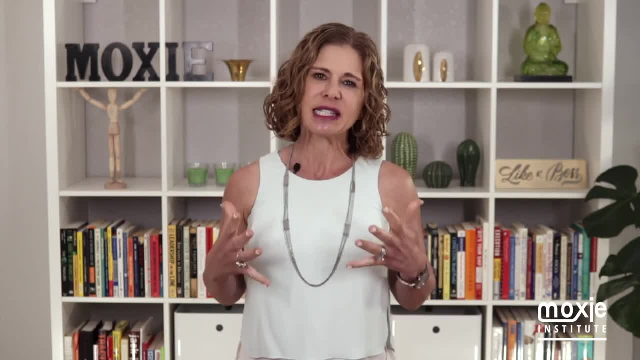 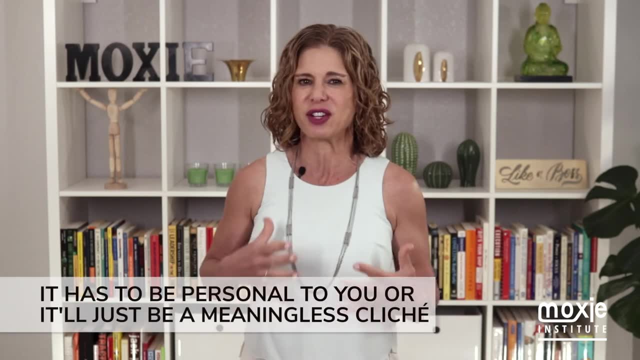 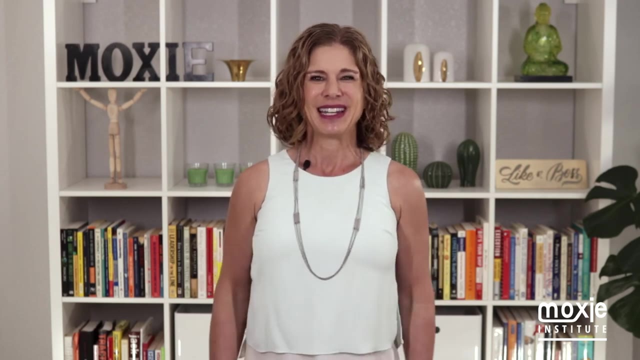 building new neuropathways. So take a stab at writing your mantra and, once you get it right, put it everywhere on sticky notes: in your phone, in your journal, in your office, and say it aloud for power, especially before those presentations. Now I want to end by saying that we can learn a 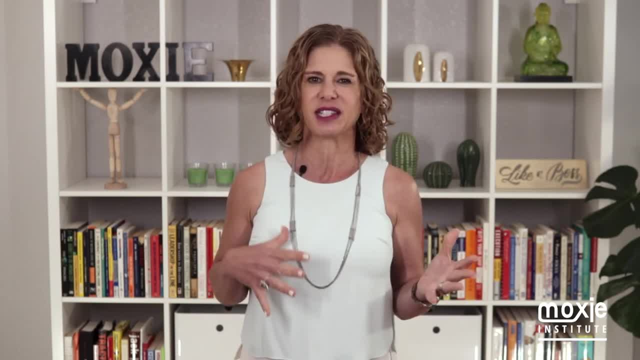 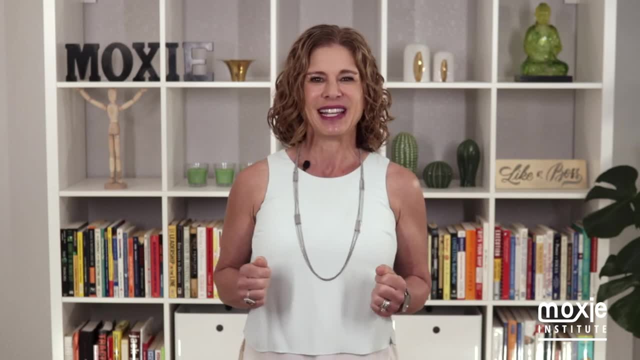 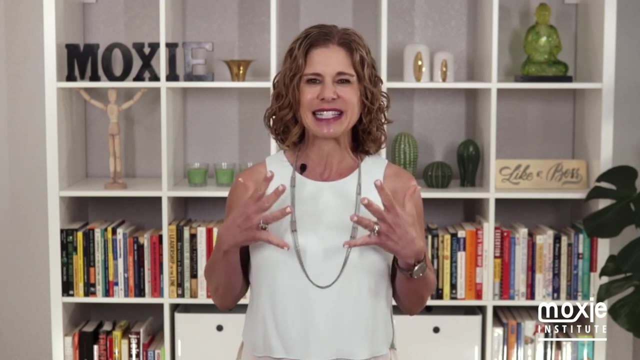 lot by taking a page out of the playbooks of top athletes and sports psychologists and performers. All of these people feel the fear and do it anyway. They learn to channel their nervous energy into usable energy And they know that the nerves are just a sidekick to doing something that matters. So next time you're.